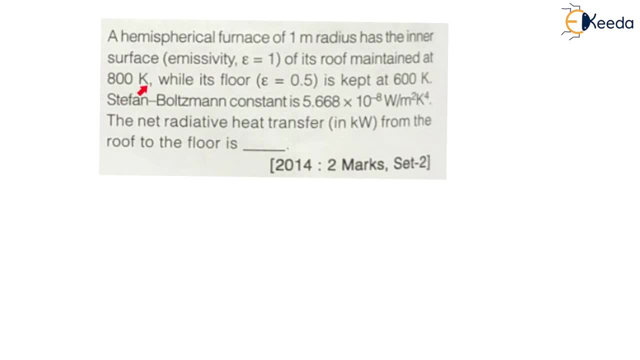 of its roof, maintained at 800 Kelvin. Now let us draw the hemisphere. If I draw here hemisphere Now, my dear students, the hemisphere will be like this: This will be the hemisphere: Half football, We can say half football, This is a hemisphere. 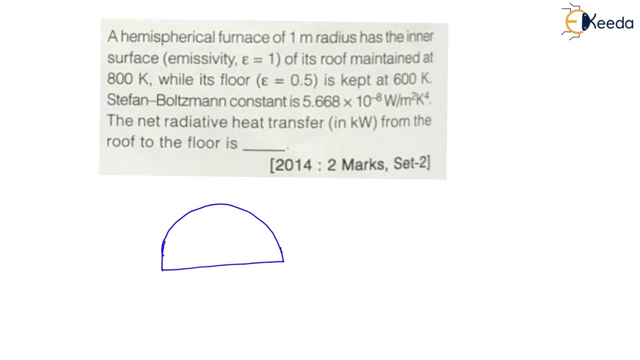 My dear students, here they have given the roof is maintained at. This is a roof, This curved surface is a roof. Therefore, let us say, This curved surface, which is a roof, is maintained at, If I say this roof as 1.. 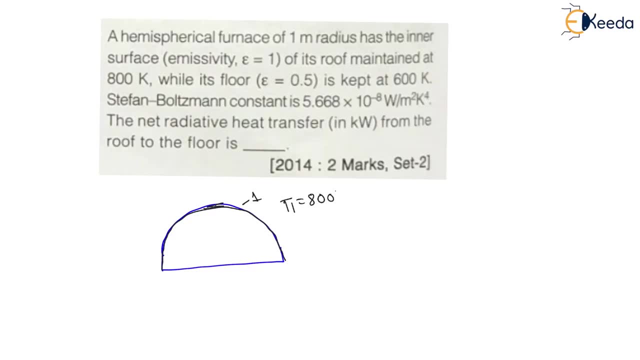 It is maintained at temperature. T1 is equal to 800 Kelvin And emissivity E1 is equal to 1.. They have given here in the question, While its floor emissivity is equal to 0.5 is kept at 600 Kelvin. 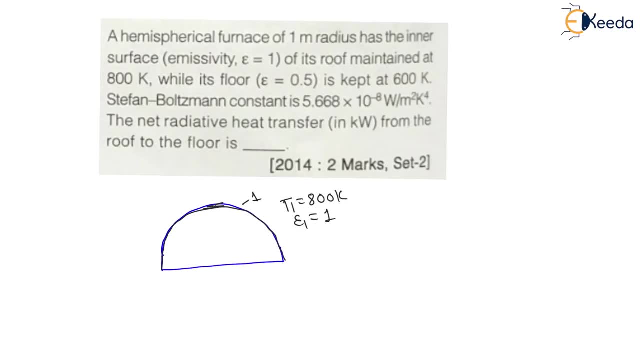 And this is a floor Now. so, my dear students, let us say here, this is a floor. I will say: the floor is 2.. Floor is 2.. And temperature T2 is given, 600 Kelvin, And emissivity 2 is also given. 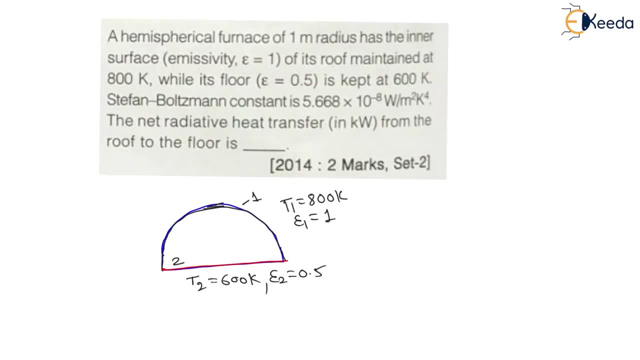 Which is 0.5.. Right Here Now Stefan-Bohlmann constant is. Now this is a sigma. The Stefan-Bohlmann constant sigma is given 5.668 into 10 to the power minus 8 Watt per meter square, Kelvin power 4.. 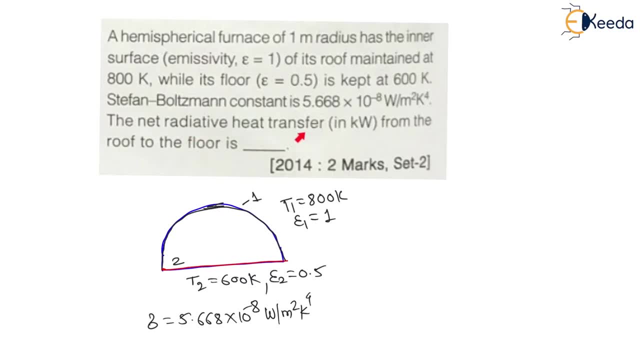 Right, Then the net radiative heat transfer in kilowatt from roof to the roof, From roof to the floor. Now, from roof to the floor, Right, What is the net radiation heat transfer? Therefore, can I say: from roof to the floor? 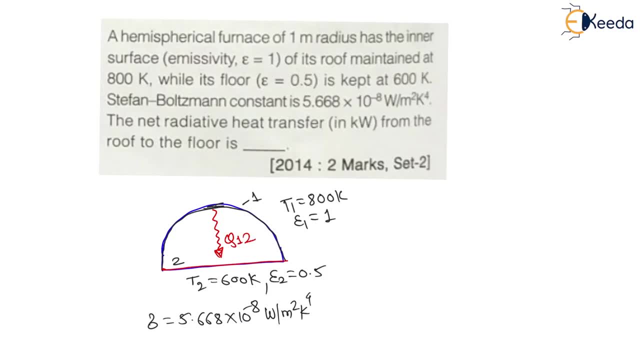 It is from 1 to 2. Q1 to 2.. So here they are asking: what is Q1 to 2.? Q1 to 2 in kilowatt? we have to find Right, So let us solve this question. 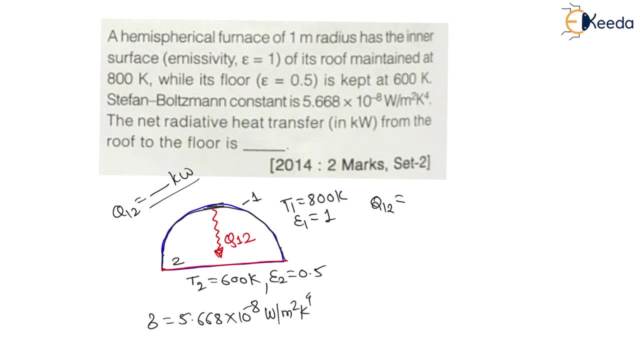 Now, my dear students, if I want to find Q1 to 2, we have one equation that we have derived in the theory lectures, That is: Q1 to 2 is sigma T1 power 4 minus T2 power 4 divided by 1 minus emissivity 1. divided by area: 1- emissivity 1. 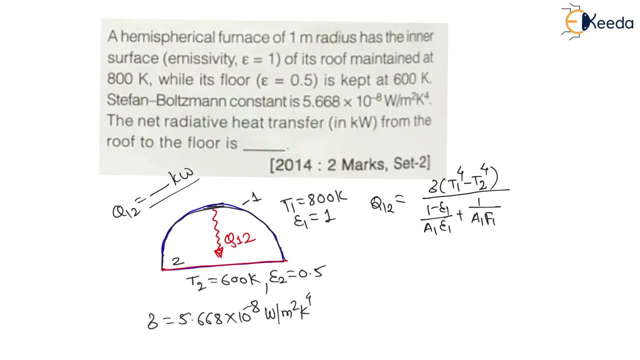 plus 1 upon A1, F1 to 2 plus 1 minus emissivity 2, divided by area 2, emissivity 2.. This expression we have derived in the theory lectures, Right. So, my dear students, if I want to find the net heat transfer from 1 to 2,. 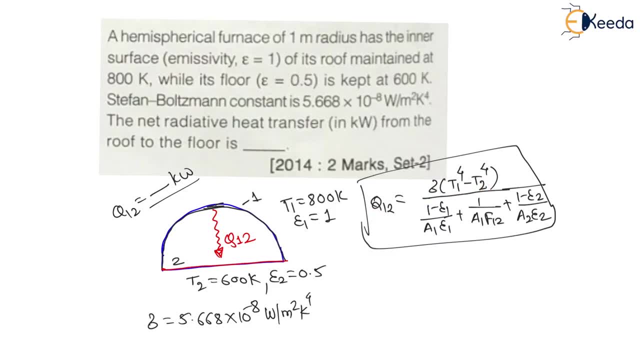 then I have to find temperatures- Stefan-Buhlmann, constant, already given. I have to find areas So we can find areas over here. We have to find emissivities and safe factor of 1 with respect to 2. F1 to 2 also we have to find. 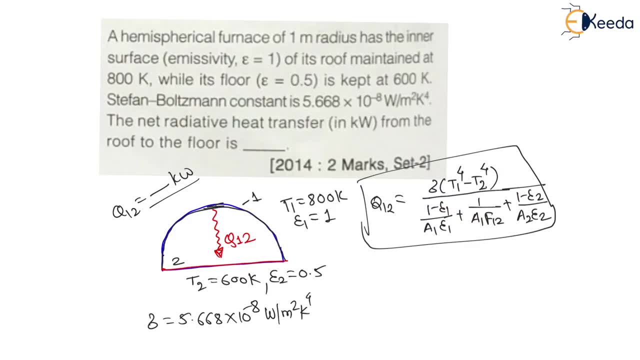 So let us find the all given conditions Now. emissivity 1 is given, emissivity 2 is given, sigma is given, T1 is given, T2 is given. Now let us find areas: Area 1 and area 2.. 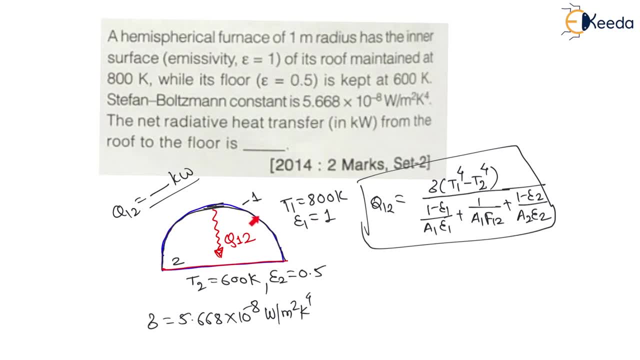 Now for radiation heat transfer. the surface area of this hemisphere, that is roof. let us say the 1 is roof. Right, This is, we can say, roof. Now for this roof. the inside surface area is in contact with this floor. 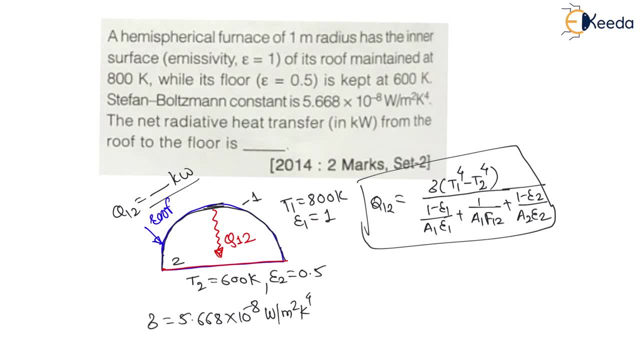 Right. Therefore, here the area 1, we can say area 1 is a half of a spare area, That is, 4 pi r square divided by 2. Right, Which is nothing but 2 pi r square, 2 pi r square. 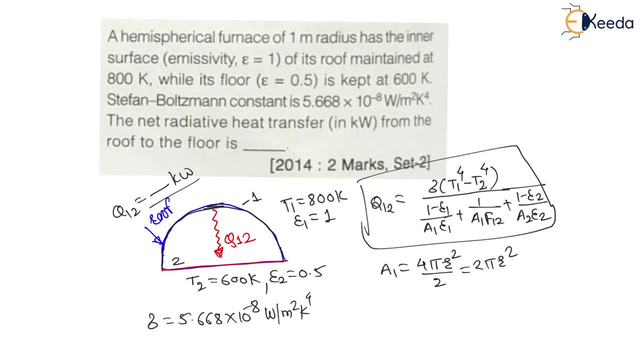 This should be the area Now for this floor. that is, surface 2, floor is nothing, but as it is hemisphere, the floor will be here circular. This should be the circular, like this. This is a floor, Right, It is a circular. 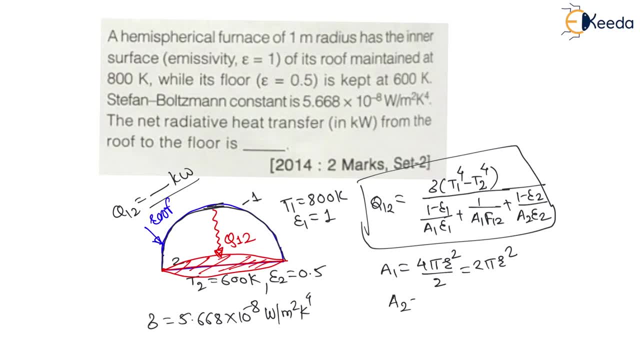 Right. So, my dear students, the area 2 will be. area 2 will be pi r square, the area of circle Right Now. here I have calculated areas, both areas Right. Let us find here 1 to 2.. 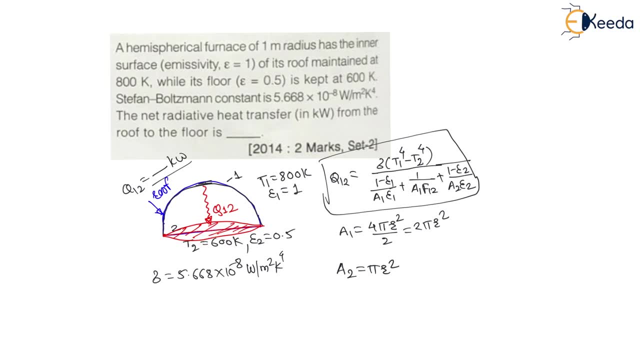 Now, my dear students, this 2 to 2 is a flat surface. Therefore, the safe factor of 2 with respect to itself, f 2- 2, will be equal to 0.. Or flat surface safe factor is 0.. 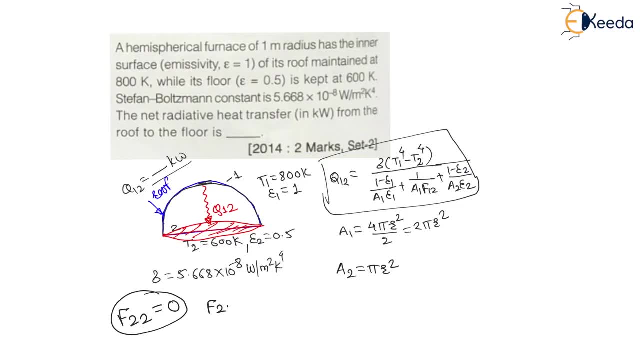 Now the addition law of the safe factor, that is, f 2 to 1 plus f 2 to 2 is equal to 1.. Therefore, f 2 to 2 is 0. Therefore, can I say f 2 to 1 is equal to 1.. 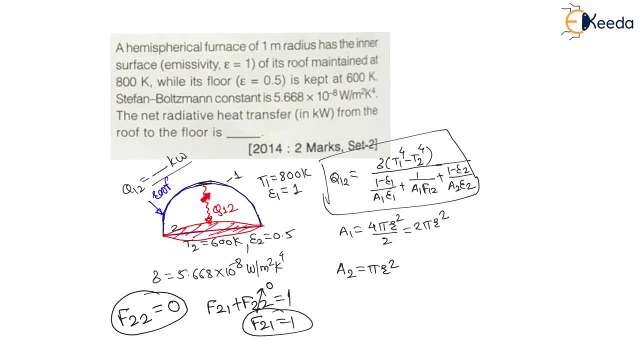 Now, with the help of this value, f 2 to 1 is equal to 1,. let us use reciprocal theorem now. Now we have reciprocal theorem, that is, area 1, f 1 to 2 is equal to area 2,. 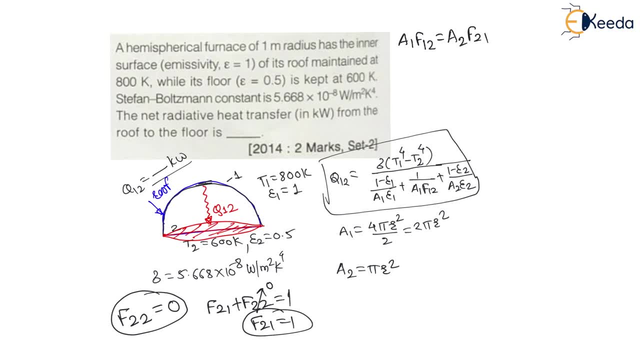 f 2 to 1.. Therefore let us put here: area 1 is 2. pi r square f 1 to 2 is unknown- is equal to area 2: is pi r square f 2 to 1,. 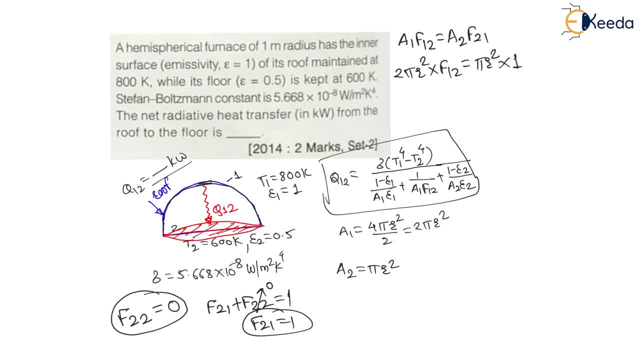 just now we have calculated equal to 1.. Right, Here we have calculated. Therefore, here pi r square, pi r square will get cancelled. Therefore, we will get: f 1 to 2 is equal to 1 by 2,. 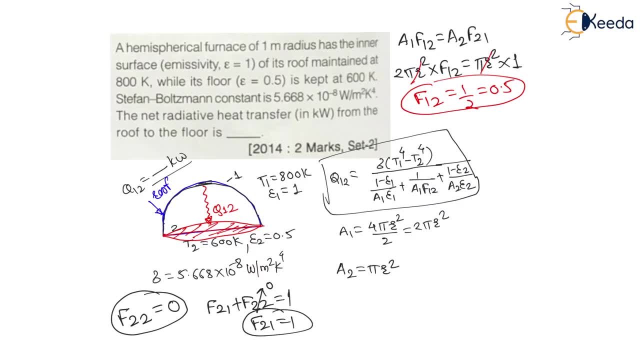 which is nothing but 0.5.. And this f 1 to 2 is required in this formula. f 1 to 2 is required here, Right? So, students, areas: we have calculated. f 1 to 2, we have calculated. 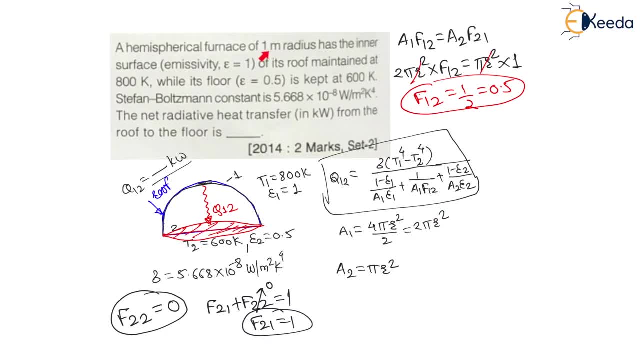 So let us use here Now for these areas the radius is given 1 meter radius. Right r is we have to use 1 meter Radius. we have to use 1 meter Right Now. let us use the formula and put the values. 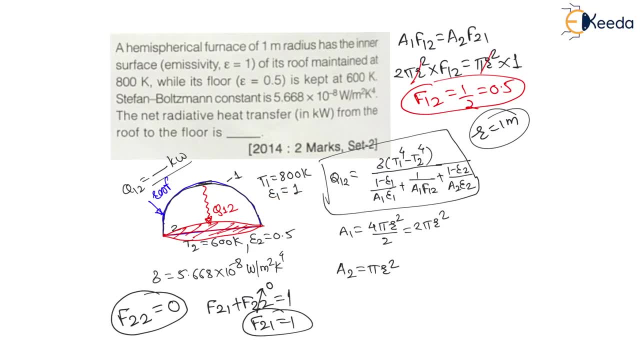 Now here emissivity 1 is given 1.. Emissivity 1 is equal to 1.. Therefore, 1 minus 1 will be 0. Therefore, this term becomes 0.. This term completely becomes 0.. Right. 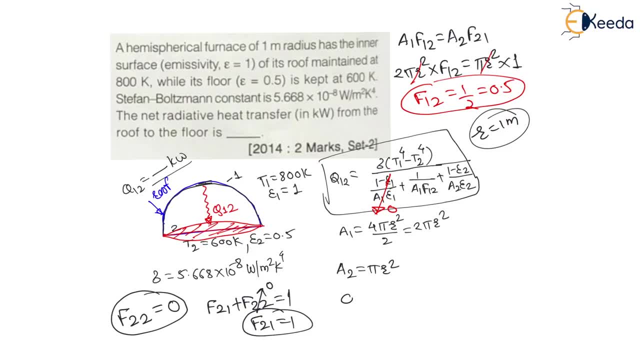 So, my dear students, the final resulting equation q 1 to 2 is equal to sigma: t 1 power 4 minus t 2 power 4 divided by 1 upon a 1 f 1 to 2 plus 1 minus. 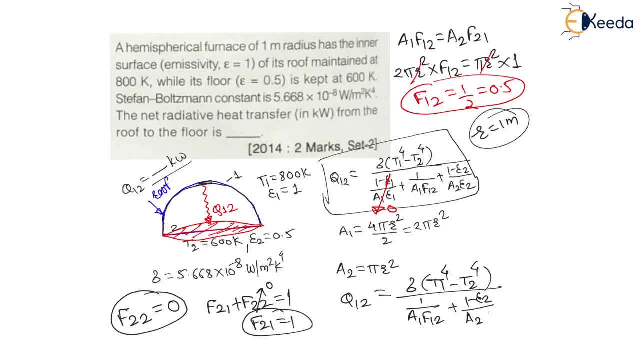 emissivity 2. divided by a: 2, emissivity 2.. Right Now, let us put the values. Now, my dear students, I am going to put here values. Now, all the values we have calculated, let us put them. 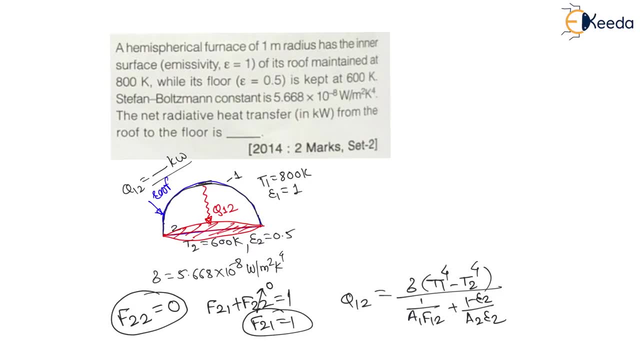 Therefore, my dear students here, the resulting equation will become here: q 1 to 2 is equal to Stefan-Bohlmann. constant is 5.668 into 10 to the power minus 8, 10 to the power minus 8. 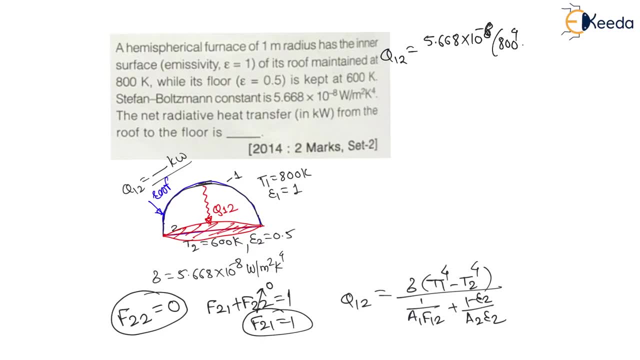 into: t 1 is given 800 power 4 minus t 2 is given 600 power 4 divided by 1 upon a 1.. a 1, we have calculated 2 pi r square right. This is the a 1.. 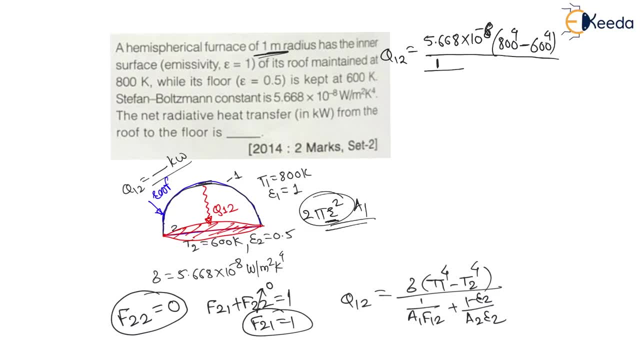 Therefore, radius, we have to put 1.. Radius, we have to put 1.. Therefore, pi into 1, square into 0.5 plus 1 minus emissivity. 2 is given here: 0.5, 1 minus 0.5. 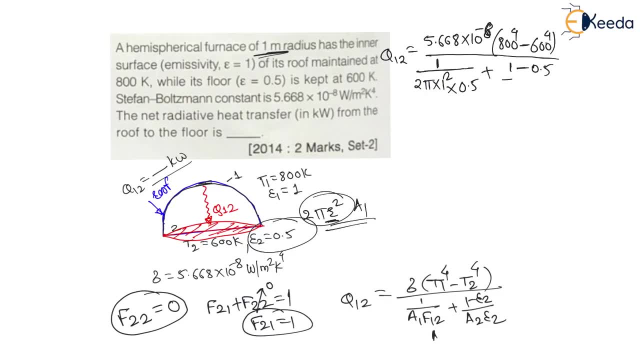 divided by a, 2. a 2 we have calculated as pi, r, square radius we have to put is equal to 1.. Therefore, pi into 1, square into emissivity 2, is 0.5. right Now, my dear students, 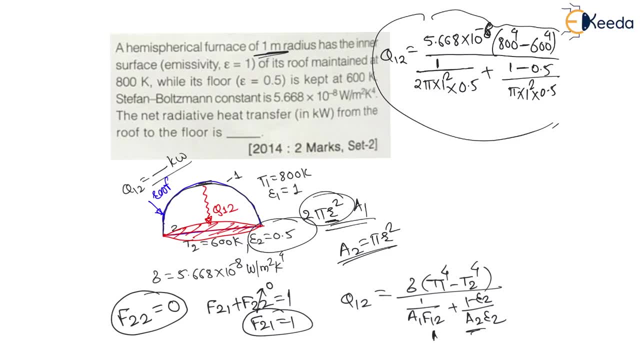 in this complete equation. let us solve this complete equation for q 1 to 2.. Therefore, my dear students, this q 1 to 2, in this equation, you will find as 24916.528 watt. This answer will be in watt. 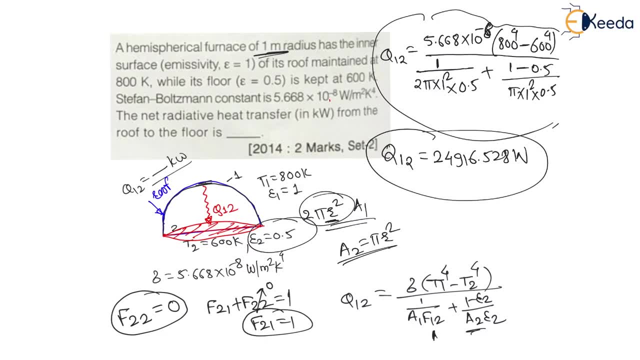 But here this is not your answer, because they are asking in kilowatt in the question. Therefore, if I divide this answer by 1000, the unit will become kilowatt. Right, Therefore, q 1 to 2 in kilowatt. 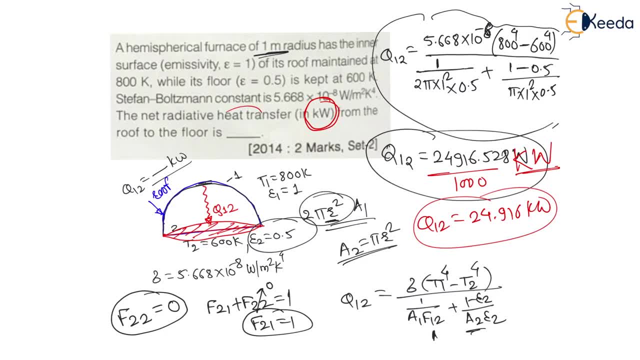 will be equal to 24916 kilowatt. So, my dear students, here in the fill in the blank, you have to type 24.916 for getting full 2 marks. Thank you, dear students. In next lecture we will see one more. 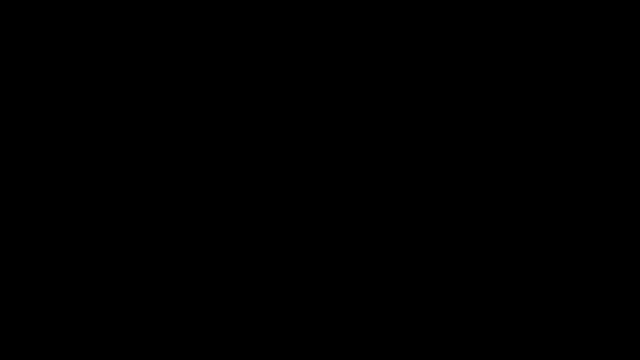 numerical on this topic, which was asked in previous year gate examination. Thank you.